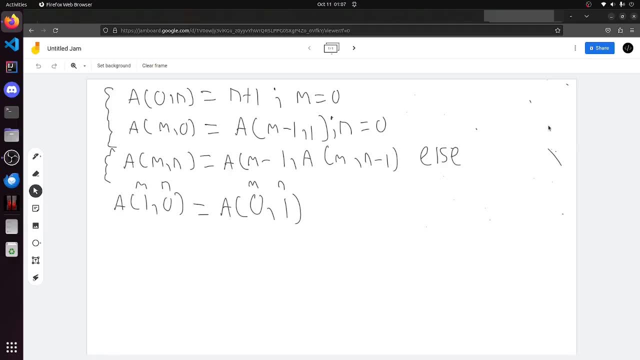 so in this case we just do n plus one. n is one, one plus one is equal to two. that's the answer for ackerman: one comma, zero. now another example, or a good example, could be: solve for: solve for ackerman: one comma, one, right. so neither m or n is zero. so we could use this equation right here. 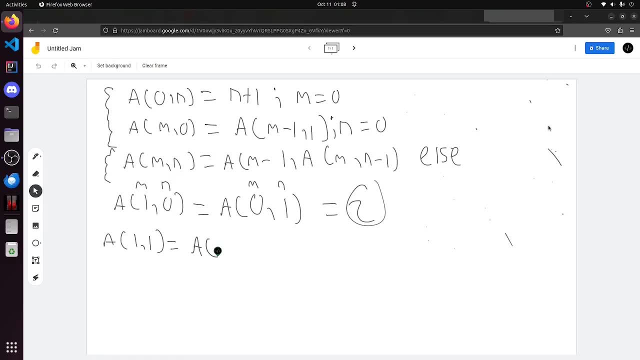 so, plugging in, we get ackerman m minus one. m is one. one minus one is zero comma. ackerman m is one: n minus one. n is also um one. so one minus one is zero is comma, zero. right and, as you can see, right we have an. 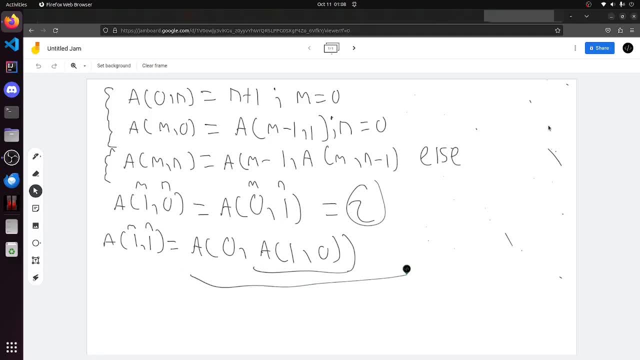 nested ackerman function within a bigger one, so in that case you always work from the inside out. so work from this inner ackerman function right here and we apply a formula to it. so this is m, this is n, so n is equal to zero. we can use this function. 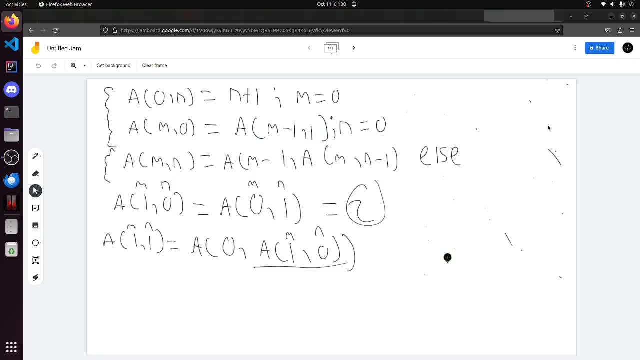 now we're gonna get- let's rewrite it below, right here: ackerman, zero comma, and solving for this right here using this formula: we get m minus one, right: one minus one is zero. so we get um: ackerman: one minus one is zero comma one. okay, now we keep on solving ackerman, zero, comma one. this is m and n. m is equal to zero. 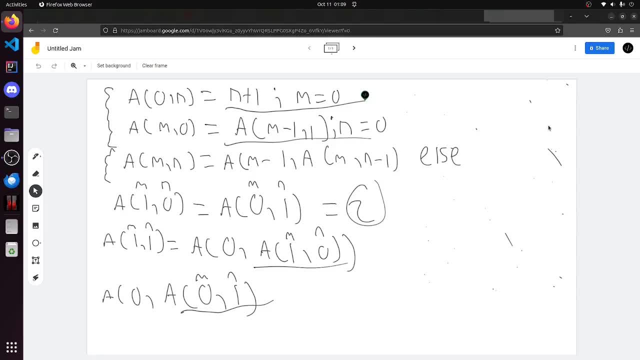 so this time we could use this equation, so that's just n plus one, which is two. so now we get ackerman zero comma two, solving again m and n. m is zero. so we could use this equation. so we could just do n plus one, and it's two. two plus one is equal to three. 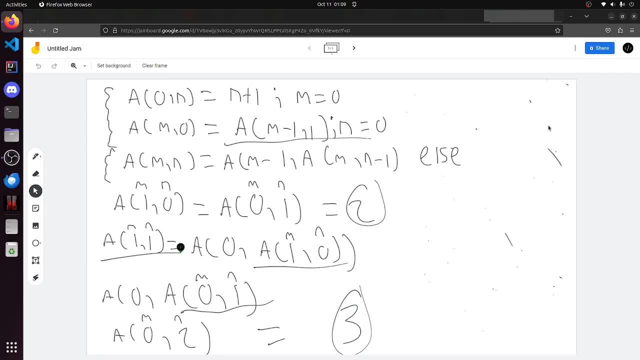 that's our answer for ackerman, one comma one, and that's just like an example of how to solve simple ackerman problems and functions.